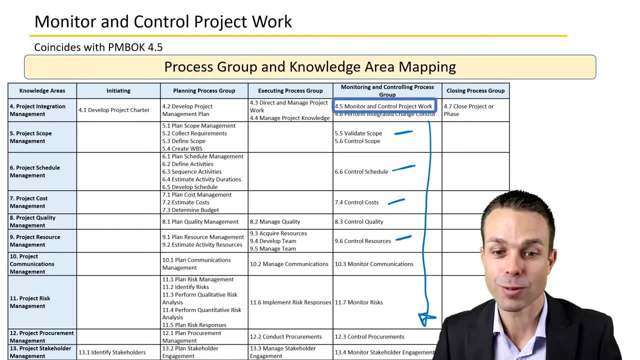 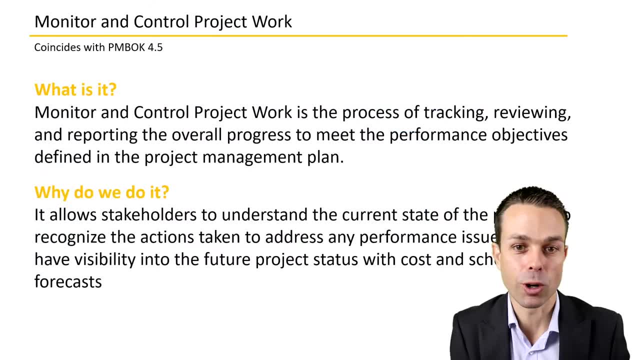 Controlling our resources to make sure that we've got the right resources for the job, and a lot of other things as part of this overall process. group Monitoring and controlling the project work is the process of tracking, reviewing and reporting the overall progress of the project to meet the 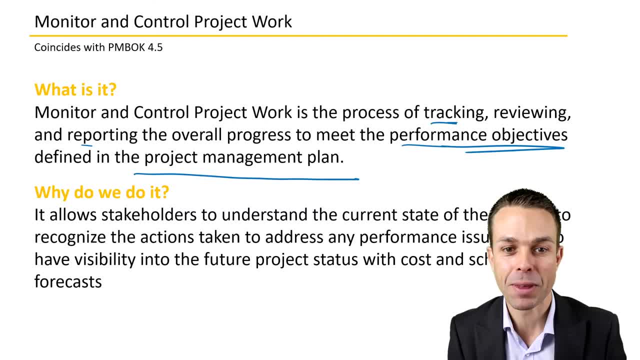 performance objectives defined in the project management plan. Of course we're coming back to that project management plan, which is our overall plan. that gets updated over time, So it's sort of an iterative document you might say. We're updating it, make sure, if something needs to be changed, changing it and putting it back into the project. 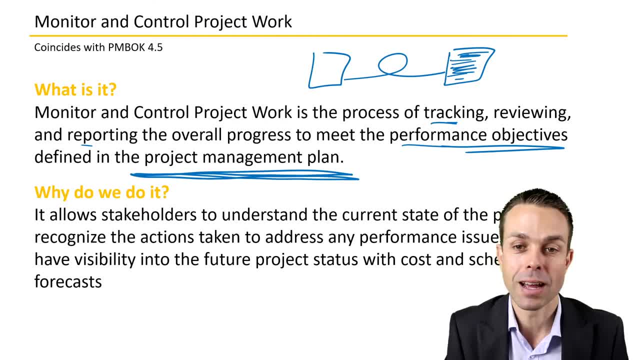 management plan. But we're monitoring that work as it goes along to make sure that it still meets what we set out in that original plan And it allows stakeholders to understand the current state of the project, to recognise any actions that have been taken to address any performance issues, like any costs going off course schedule going off course scope. 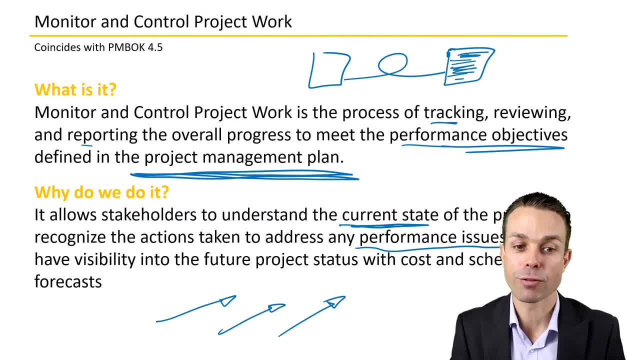 needing to be changed And to have visibility of into the future project status. So if it's going off course now, maybe it's going to go off course in the future, for example, and we want to steer that back on course and you know, need to take the corrective actions appropriate at the time And so future. 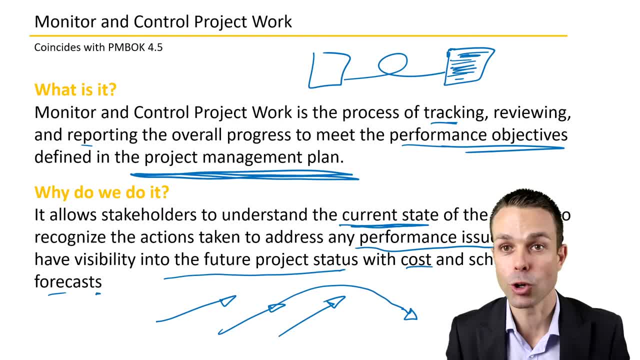 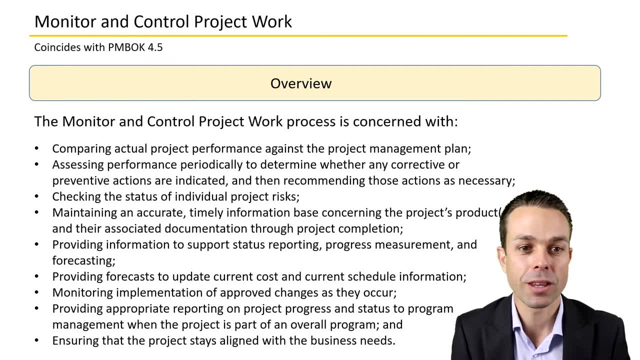 project status, with cost schedule forecasts and, of course, scope and quality is involved. there, too, An overview of this particular process is it's: this process is concerned with comparing the actual project management performance against the project management plan. So here's what we planned And here's where we are, And so maybe we want to bring ourselves back down to where we had planned. 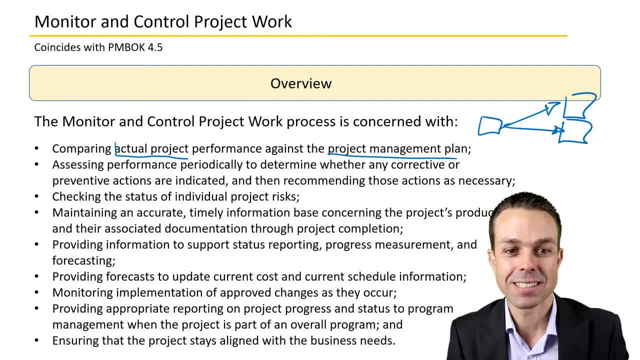 or where we wanted to be at this point in time. We're assessing the performance periodically to determine whether any corrective or preventative actions are need to be taken And sometimes, if those actions need to be taken, that is a change request that goes through the change control board as part of the change management plan. All of these things are starting to tie. 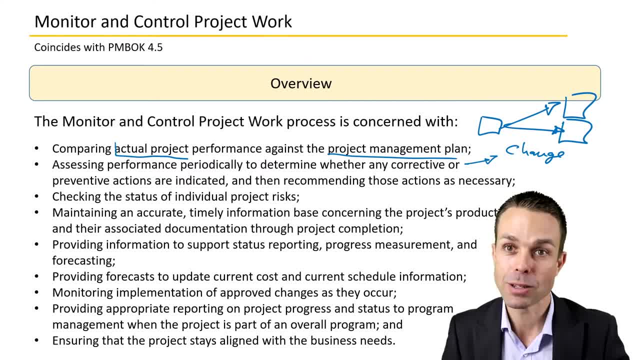 together. There is definitely a lot to remember, but you'll see them come up time and time again for the reasons that they use in the project management plan. We're checking the status of individual project risks. We're maintaining an accurate, timely information base. 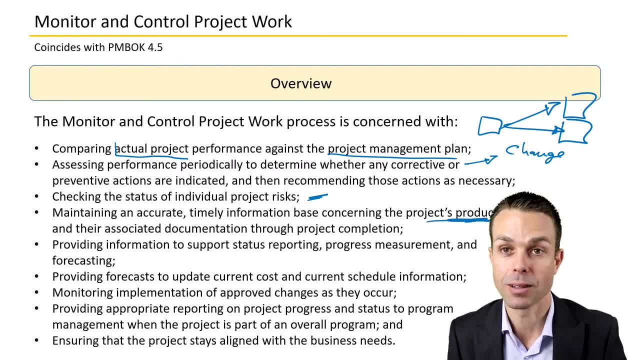 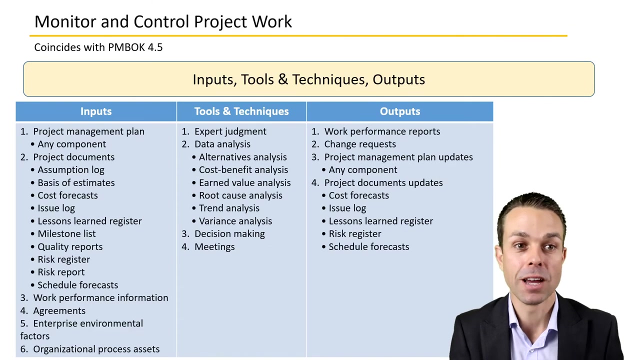 concerning the project's products. Are those products accurate? Are they going to be delivered in the right way for what the customer wants? Providing information for forecasting, forecasts for cost and schedule information, monitoring implementation of approved changes. Then we more more as they occur. if we need to make a change, Then we make that change. How's that gone? Is that the way that we wanted? We're ensuring that the project ultimately stays aligned with the business. 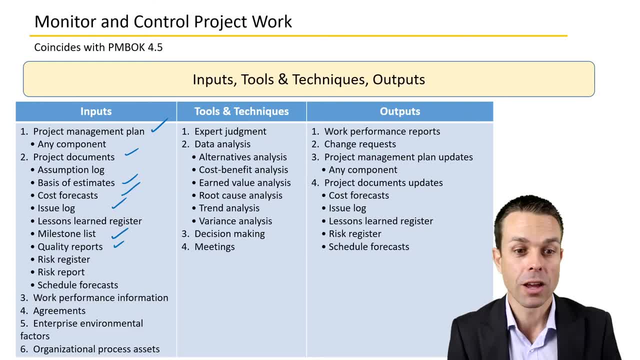 quality reports, milestone lists- all of those things work performance information- how has our project tracked to date? that's going to be an input to see if we need to make a change, any agreements that have been made that we need to refer to, and eefs and opas. we've got tools and 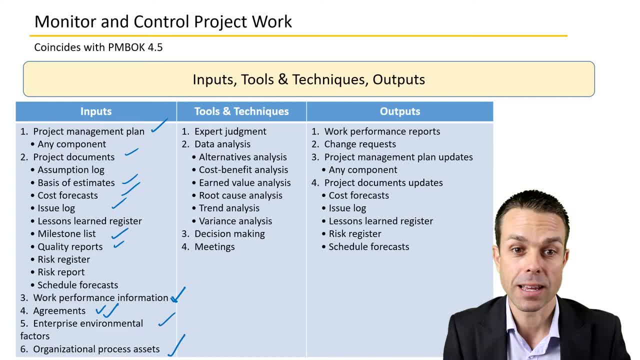 techniques that we will need to use as part of this process is any expert judgment from particular people. data analysis: so we're analyzing how the project's gone: do we need to control it or bring it back on course? decision making: we might have to make a few decisions, sometimes some tough. 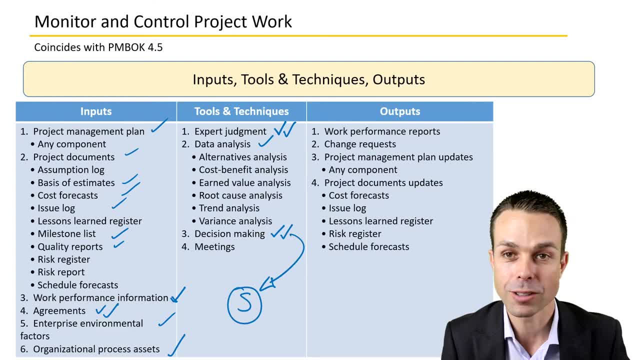 decisions. maybe a piece of scope isn't what we wanted and we need to. you know, change it and it's going to cost more. these are tough things that we have to bring back and raise the go through the appropriate processes through the change control board. make sure everyone is aware that this is. 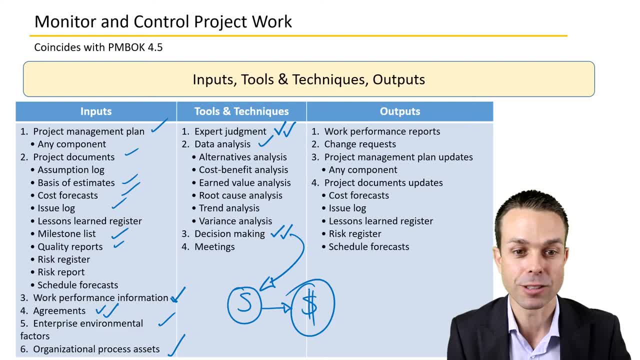 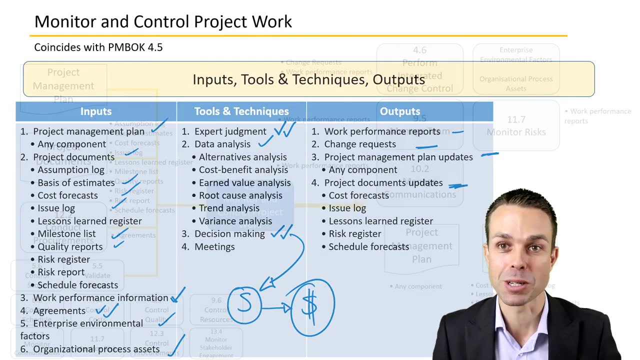 happening and, of course, meetings will help facilitate all of these things. now work performance reports are an our output. change requests might happen as well. project management plan might be updated and project management documents might be updated as an output of monitoring and controlling project work. as you can see, there are many processes that have an input into monitoring and controlling. 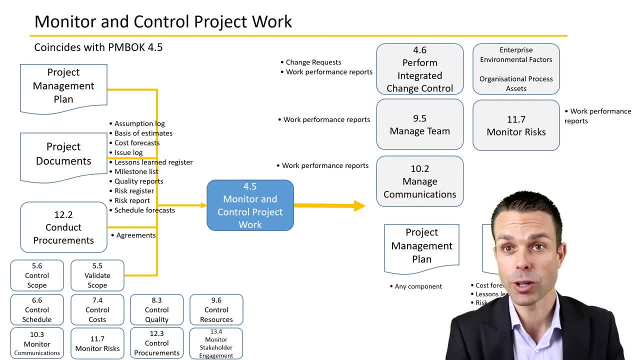 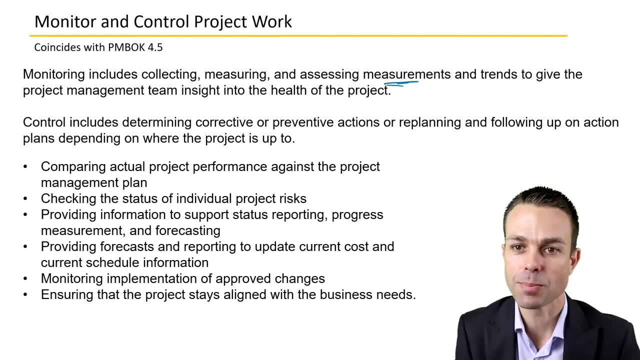 project work, which makes a lot of sense because we're executing on that work and now we're needing to monitor and control it. monitoring includes collecting, measuring and assessing measurements and trends to give the project management team insight into the health of the project. and that's where that- where that project management information comes into it- that we're going to. 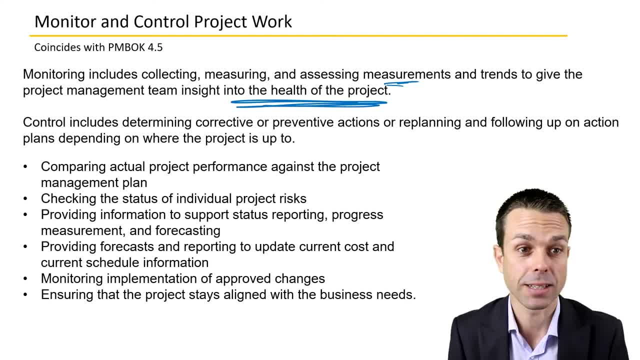 need to use to assess that and monitor those things. control includes determining corrective or preventative actions or re-planning and following up on an action plan, depending on where the project is up to. so again, it's comparing the actual or what we had planned to what is actually happening and then potentially providing forecasts based on. 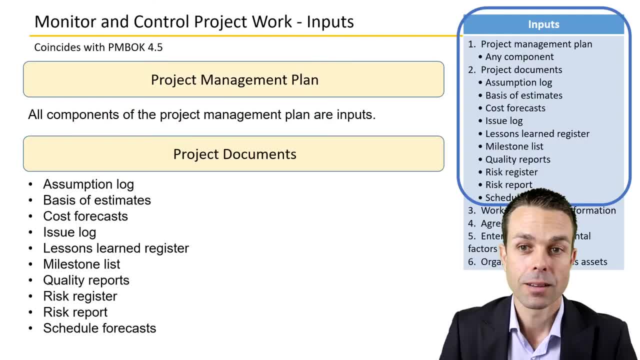 that, so that we know where we're going to be in the future as well. well, Let's look at the inputs. We've got the project management plan. All components of the project management plan will be an input into this, because we're needing to see what the plan is. 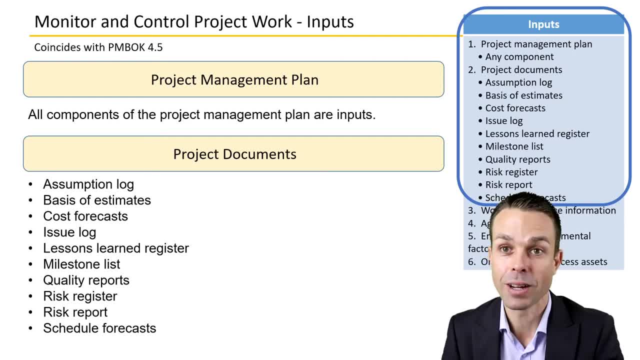 execute on that plan and then control that plan and make sure it stays on track. The project documents as well will be an input Cost forecasts basis of estimates. what did we estimate that happened and why The assumptions log. what assumptions have been made? Milestone list. 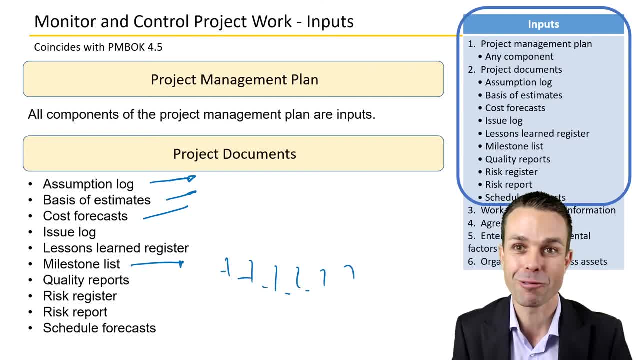 what milestones are we tracking to and have we met them so far? Quality reports. so is it a good quality for this particular item? Is it a bad quality once it's been tested, Sometimes by the front line, or the ultimate people who will be using it at the end might get their hands on it. 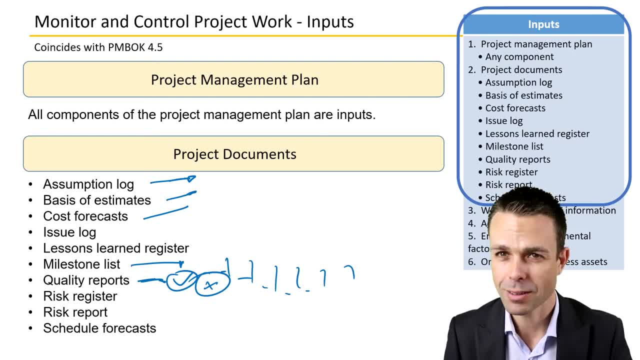 early, be able to test it and say: you know what? this isn't actually right. This isn't the way that we wanted it, So we have to go back. We need that quality report to monitor how it is tracking. Risk register- risk report. 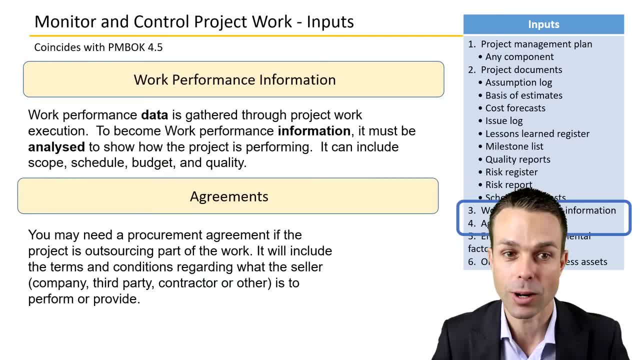 And schedule forecasts to make sure it's on track. To do that we'll need a work performance information, which is so we go in three phases. Data is the raw data, So just pure measurements. That turns into information. So this is our work performance information And that's where we're 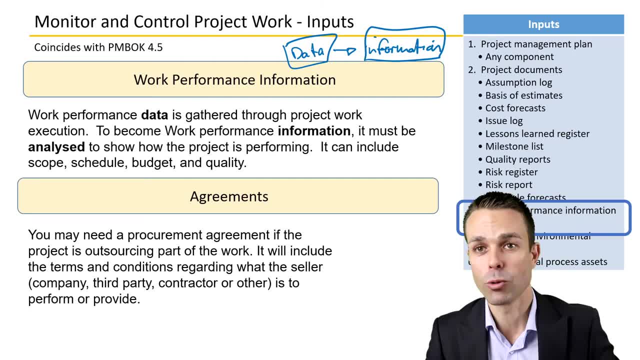 turning it into things like percentages or ratios or basically comparing it to other information so that we can show easily how something is tracking, For example the cost performance index. With that, as you'll see later on, if it's over one, we've delivered more than what we had planned, Or if it's less than one. 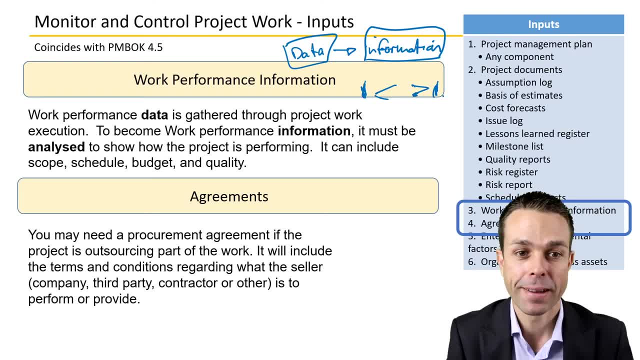 we've delivered less than what we had planned. So definitely things like that. Or we might be 80% complete or 90% complete, So that work performance data turns into work performance information And that's what we use to analyze how the project is going. 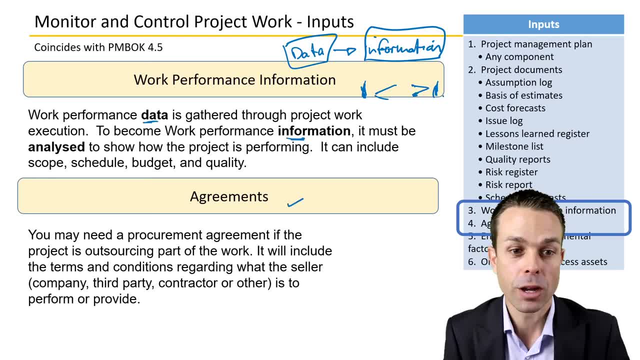 We might need agreements as well, So you might have a procurement agreement for if the project is outsourcing part of that work, And that will include terms and conditions regarding what the seller is to perform or provide as part of their contract. Of course, with EEFs and OPAs we might have 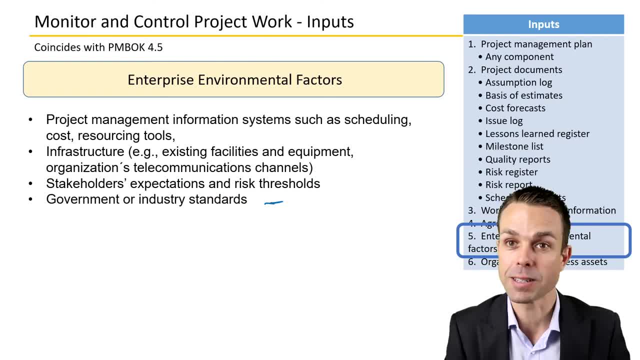 government or industry standards, stakeholders' expectations or risk thresholds. Maybe they'll have a high risk threshold or a low risk threshold- Very important to know so that we don't, you know, burn any bridges there or don't give them any box, you know, without communicating something properly. 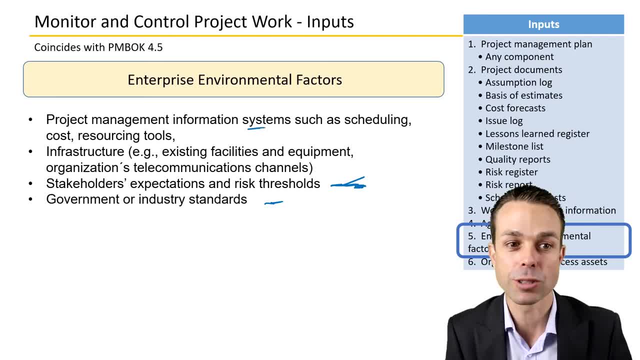 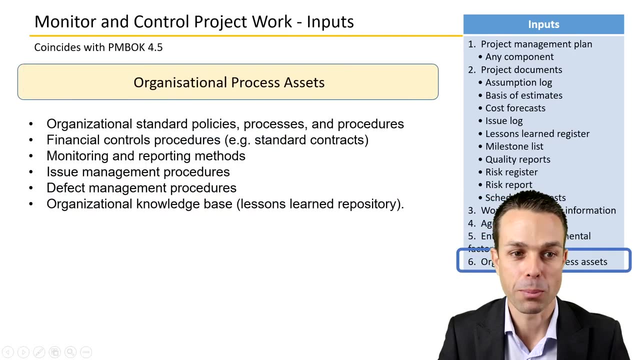 And the project management information systems, such as scheduling tools, resourcing tools, cost tools, all of those things that we're putting that project management data into so that it can turn into project work performance information, of course. And then, of course, there might be templates, specific reporting methods that you might. 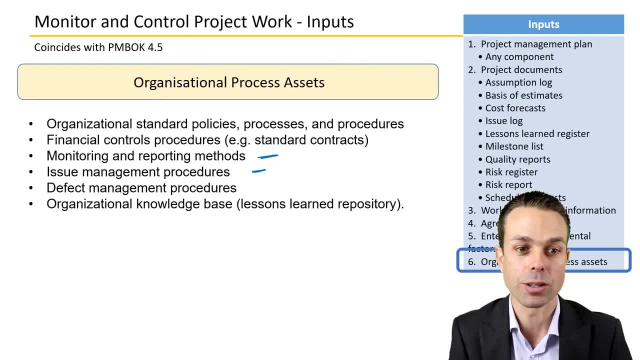 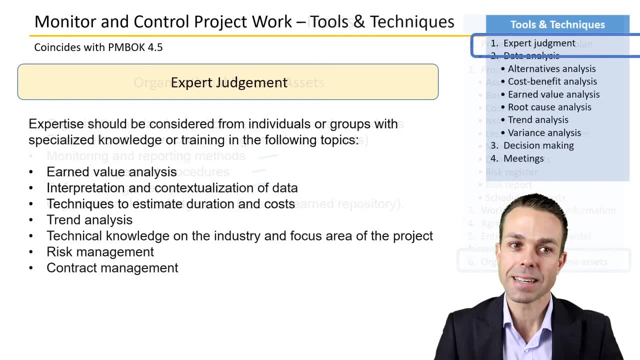 have in a company issue management procedures or defect management procedures that are already existing in the company that you're working within, that you have to abide by Tools and techniques for monitor and control project work. Of course, as you've seen quite a lot, we need expert judgment. 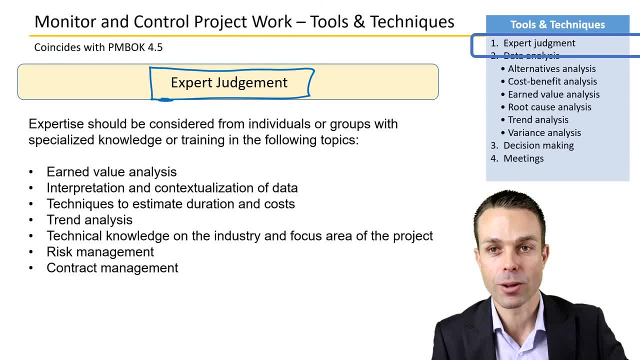 So the people who are experts in their particular area- whether it's the people who will be using the product ultimately or in other things such as risk or contracts for procurement- all of those experts you'll need to gather that information and help bring them on board. 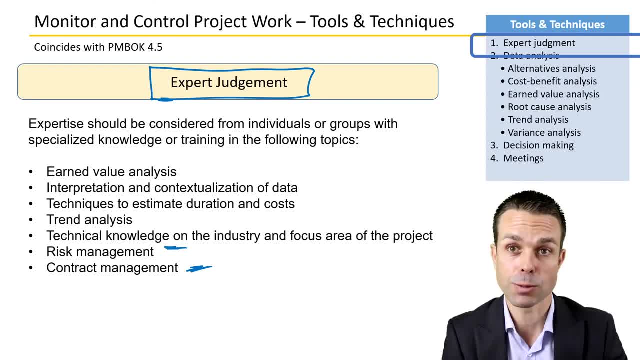 to your project to help do those things or gather that expert knowledge As needed, you might have earned value analysis. So how is the project tracking? That's where we're looking at their trend analysis. Is it trending in the right direction? Is it trending in the wrong direction? 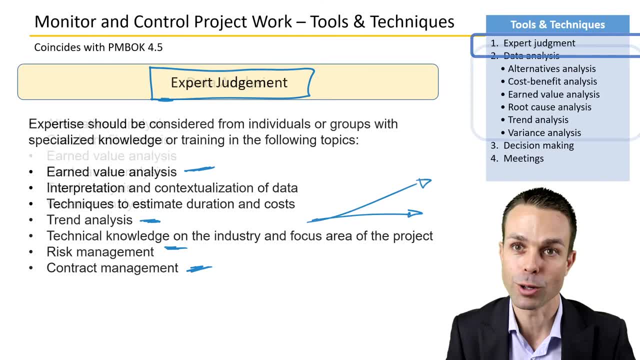 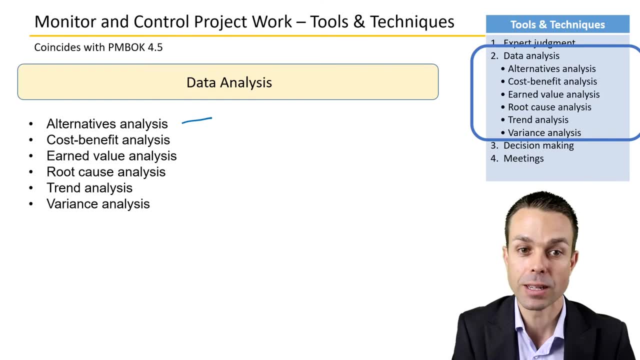 And, of course, techniques to estimate duration and costs of your project. Data analysis is an important part of this where we might be looking at different alternatives, So maybe we, if the scope needs to change or if the cost or schedule needs to be brought back on track. 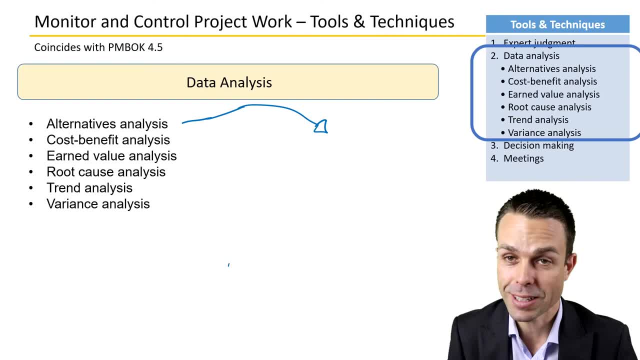 We have a few options. We might say- and you'll see these come up in future processes- We could fast track the project, And that's where we perform a few activities in parallel instead of side by side. So now they're all being done at the same time, just by different people. 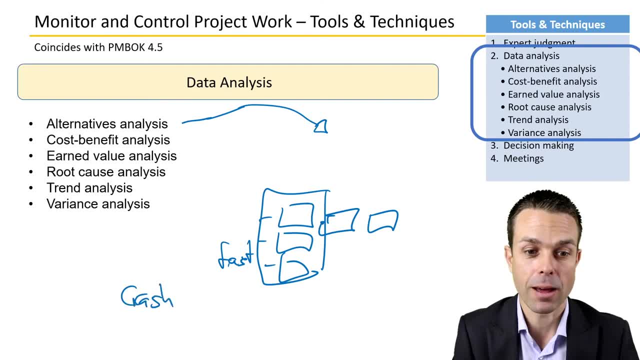 Or we could crash the project and that project schedule And that just means that we're adding lots and lots of cost and resources to try and get the job done. So there's a few alternatives and we'll need to analyze those and make a decision. 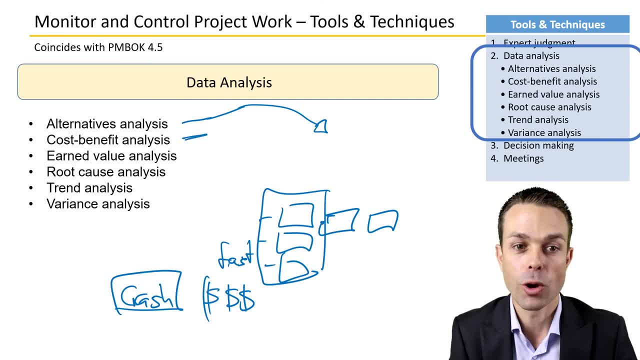 Cost benefit of those of those alternatives as well. Earned value analysis: you'll see in your cost and schedule processes. Root cause analysis of any problems that have come up: You'll see things like the fishbone diagram or the Ishikawa diagram later on in quality. 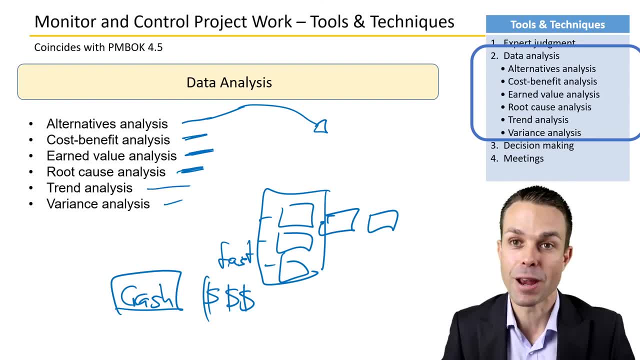 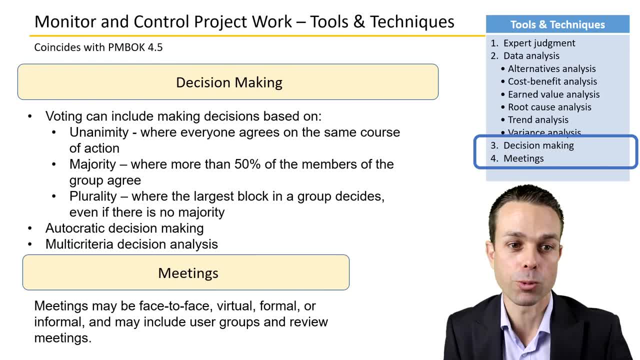 And, of course, we'll have decision making and meetings as part of the tool. So those are the tools and techniques that you'll use for monitor and control project work, And decision making might include voting on some of those outcomes that need to be to. 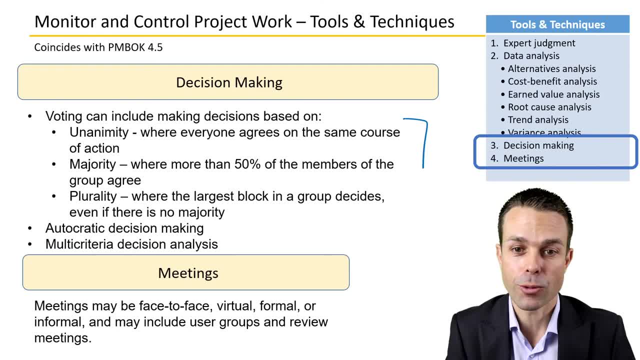 be made to have a decision on. So, when you're voting, there are three different courses of action, And you'll see this in one of the key concept videos also. But unanimity is where everyone agrees. So we've had a vote and everyone agrees on the same course of action. 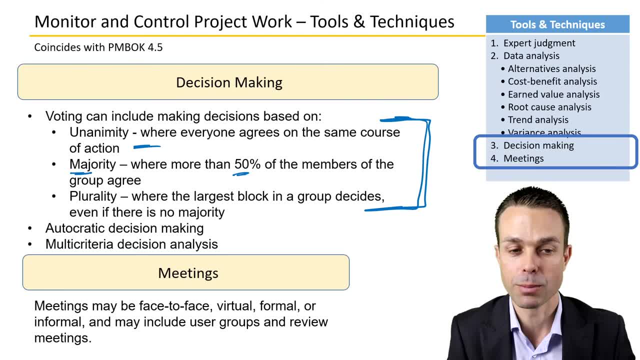 The majority is where more than 50 percent of the members of a group agree. So we've had a vote and everyone agrees on the same course of action. So we've had a vote and everyone agrees on the same course of action. So we've had a vote and everyone agrees on the same course of action. 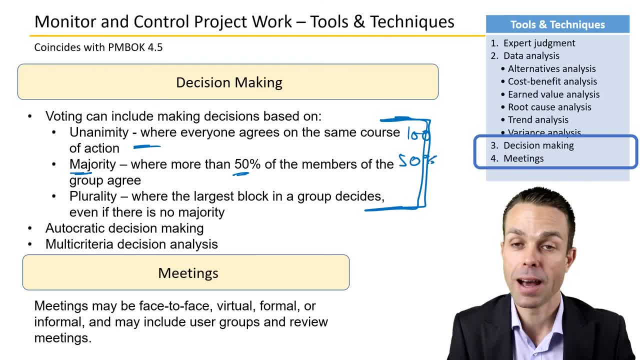 So it's not 100 percent, but it is more than 50 percent. Now plurality is the last one, and that's where just the largest block agrees, So it might be 30 percent, but then all the others are 20,, 10, 10, and 5 percent. 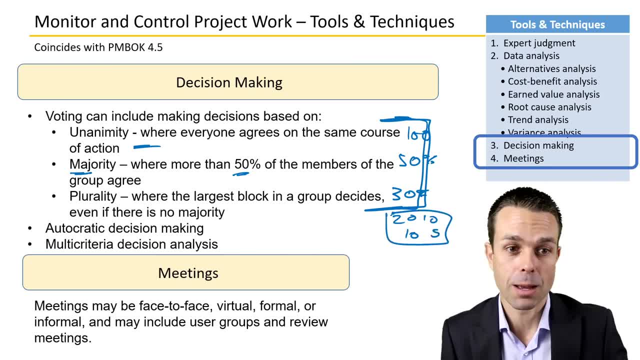 or whatever that is. So you might see that on the PMP exam also, But that's an example of voting and making a decision that way. Of course you've also got autocratic decision making, where someone, one person, just says: this is the way it's going to be. 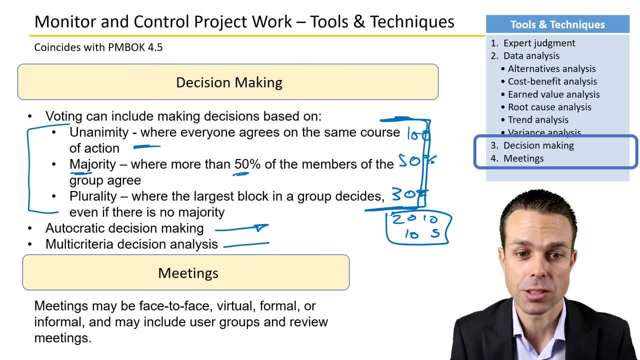 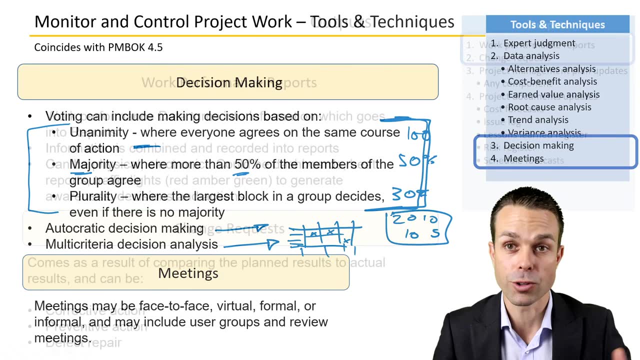 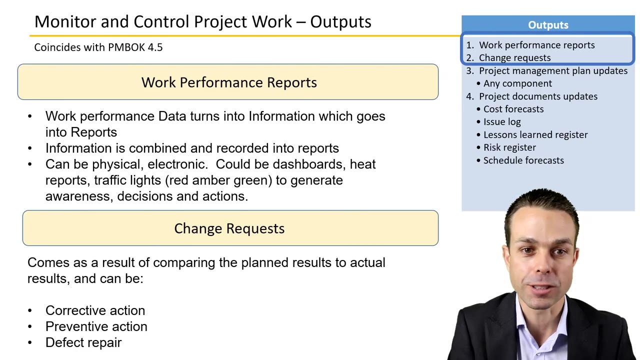 and, of course, multi-criteria decision analysis, where you might have a table of items and does it meet this criteria? does it meet this criteria? does it meet this criteria? and that will help you make the decision for the different alternatives that you have Outputs for, monitor and control project work. We've got work performance reports, So work.